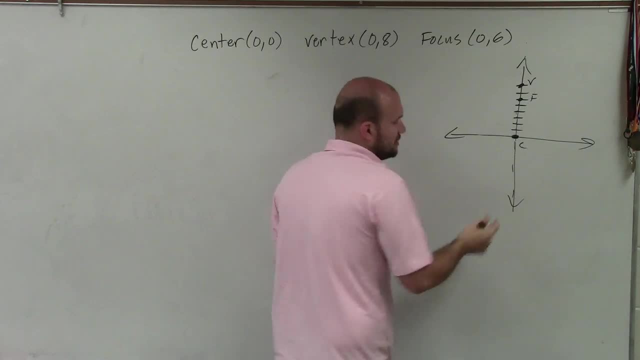 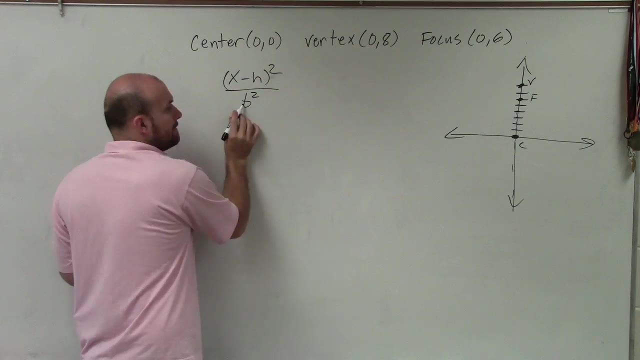 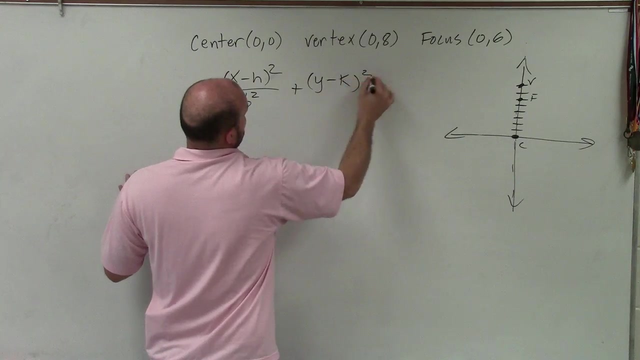 that this major axis is the y-axis And therefore it's vertical. And when it's vertical, we write the equation of the ellipse like this: x minus h squared over b, squared where b represents the distance from the center to your co-vertice, which we don't have, plus y minus k squared all over a, squared where 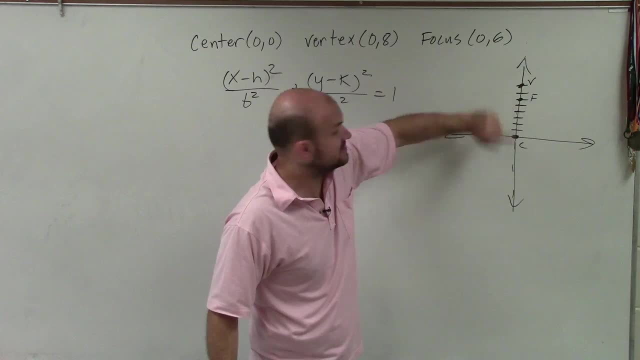 a represents the distance from the center to both vertices. Well, remember, the center splits your two vertices. So if I'm going up 7 or 8 to get to this vertex, I can go down 8 to find the other vertex. But all I really care about is this distance, which? 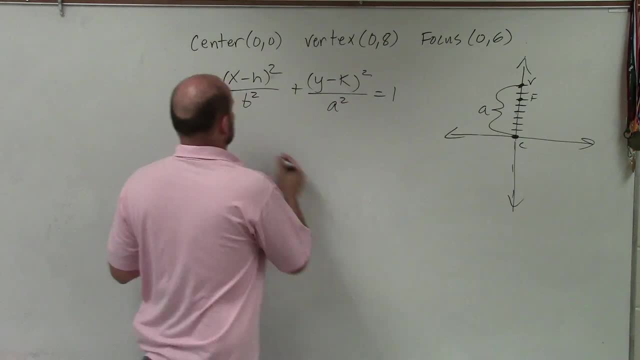 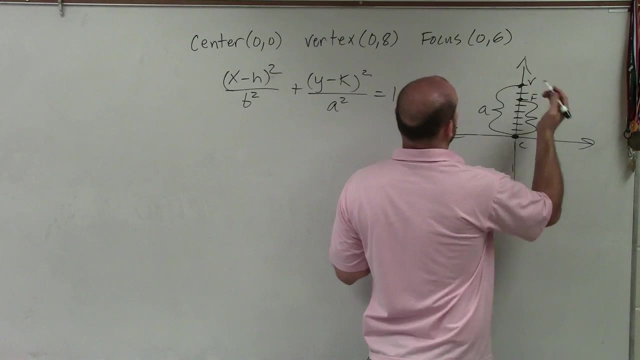 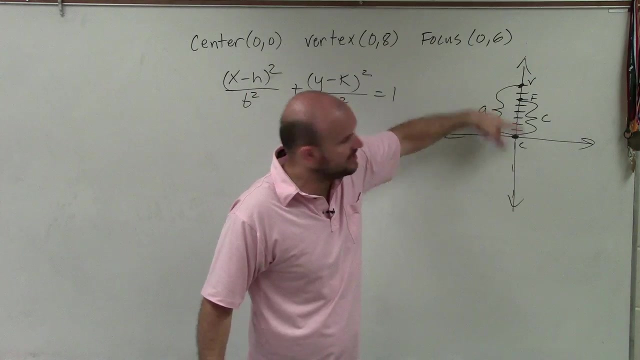 is a And that distance is 8.. So we'll get to that in a little bit. We do know that the distance from one of the foci is going to be c, And we know that distance. Again, it would be c going up and also going down, But that distance is going to be 6.. The problem is we don't 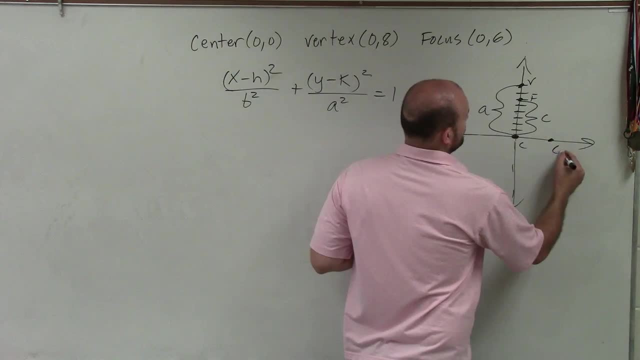 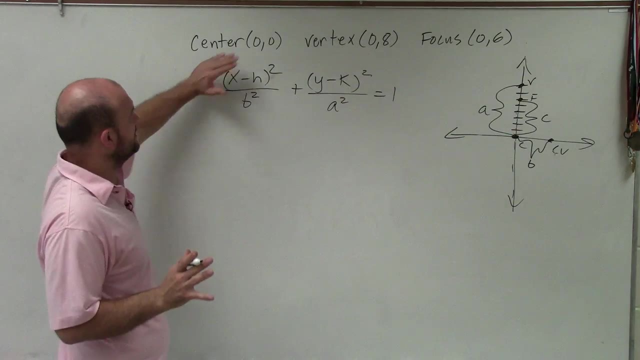 know what b squared is, And b represents the distance to your co-vertice. So we're going to have to figure that out. But before we get to that, let's look at the center. Now, remember the center we represent as hk. So since that's 0 and 0, I can say x squared. 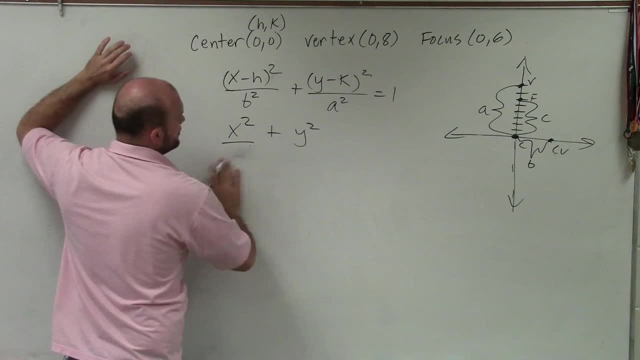 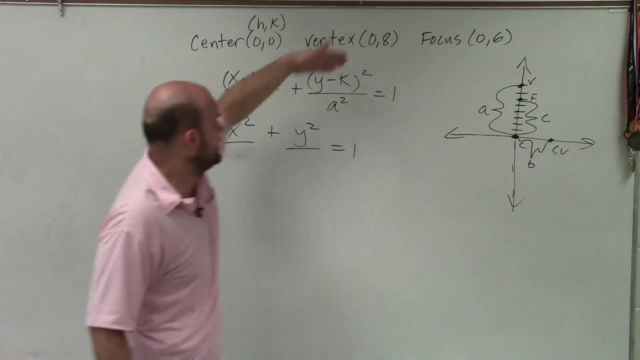 plus y squared over. let's just we don't know what b squared and a squared are. Actually, we do know what a squared is. a squared is 8, right, The distance from the center to your vertices is 8.. So 8 squared is going to be 64.. Now what we need to do is figure. 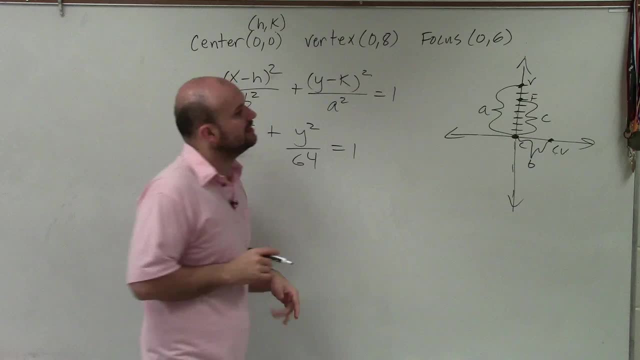 out what b is. So there is a relationship between the distance from the center to the co-vertice, which we're going to have to figure that out. But before we get to that, let's look at the center. Now, remember the center we represent as hk. So since that 0 and 0, I can say x squared plus y squared. over. we can say hk. So since that's 0 and 0, I can say hk. So let's look at the center and its and vertex, and that relationship is essentially the distance. Let's look at the center here. Let's look at the center here. Here are the distances of your center. 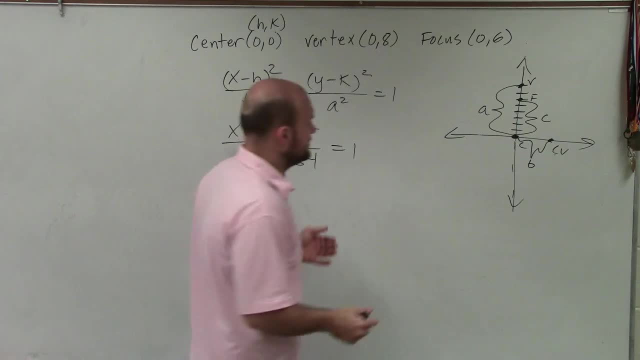 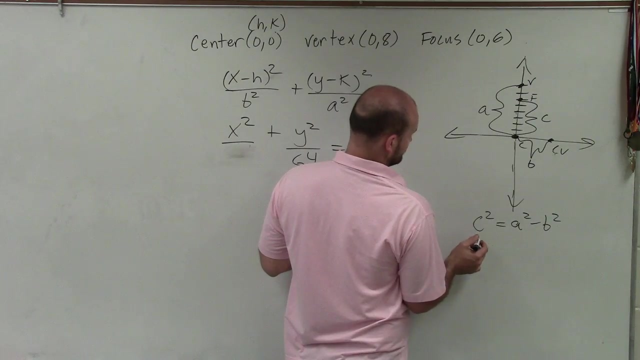 to your focus, co-vertices and vertex, And that relationship is: c squared, equals a squared minus b squared, And that relationship works for all ellipses. OK, So c squared is the distance from your center to your foci, which in this case is